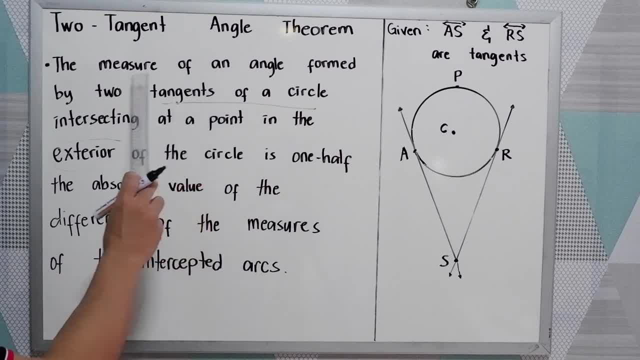 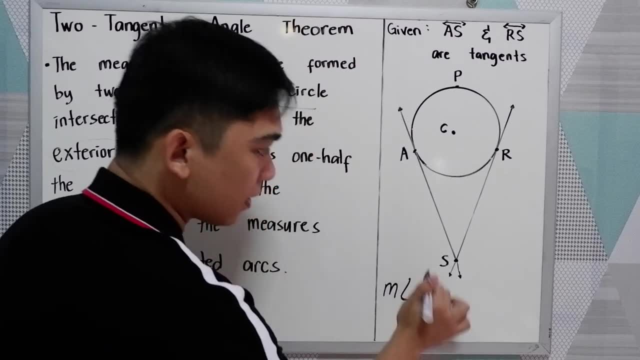 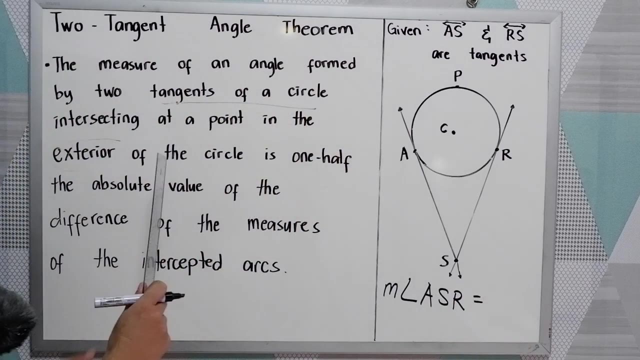 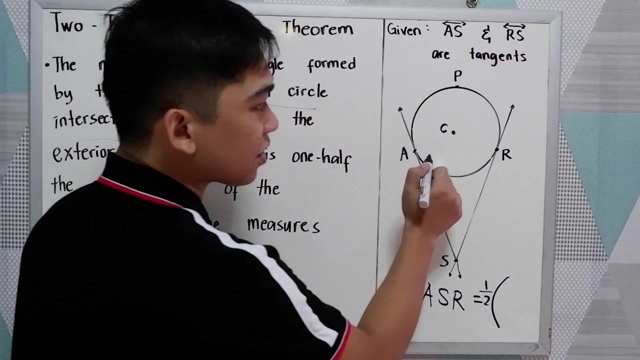 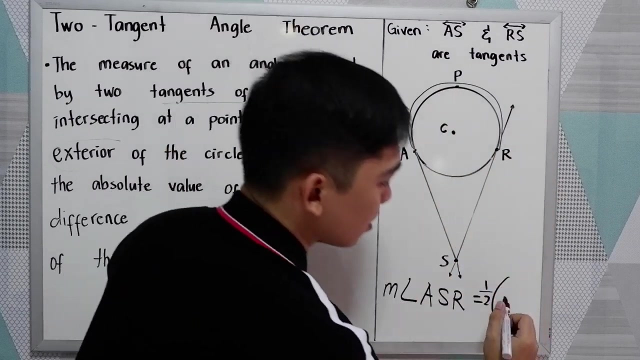 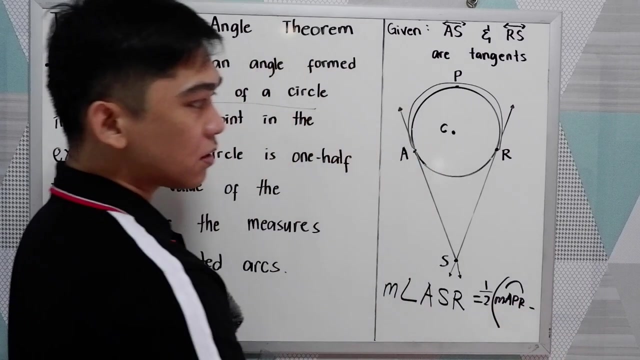 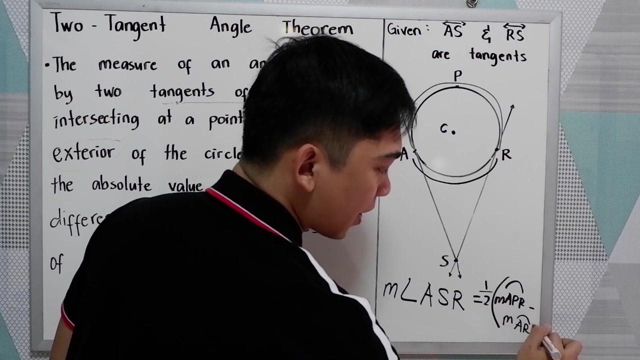 In our theorem the measure of the angle. here for our conclusion, the measure of angle ASR is one-half. One-half the absolute value of the difference of the measures of the intercepted are. So our intercepted R is APR. so we have the measure of the R APR minus the measure of R AR. 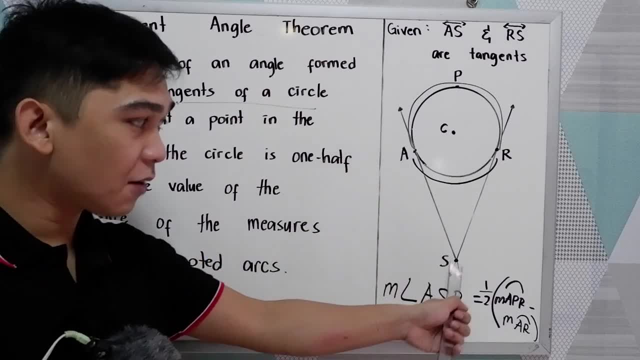 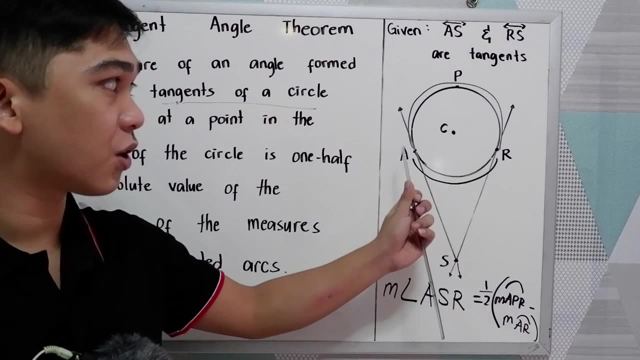 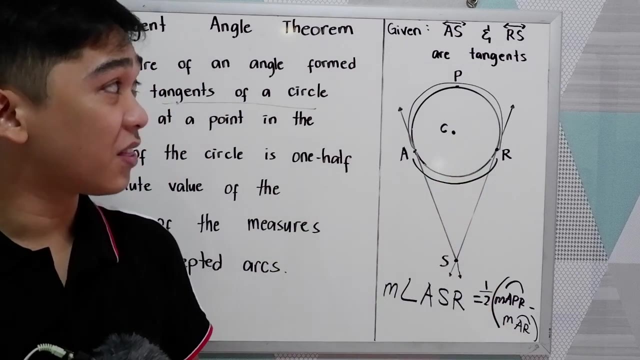 Again, let us repeat: The measure of the angle formed in the exterior of the circle Circle is one-half the measure of the intercepted R. So we have the APR minus the measure of AR. Now to better understand, let us try to solve some problems regarding this theorem. 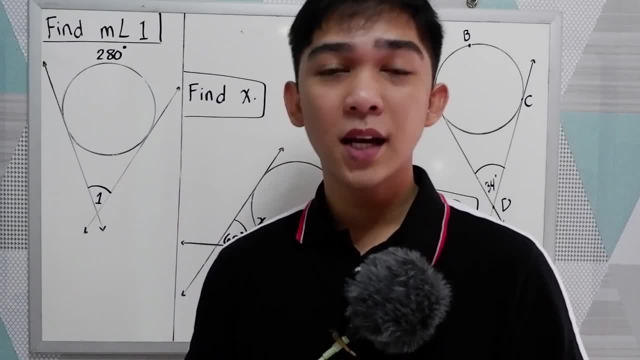 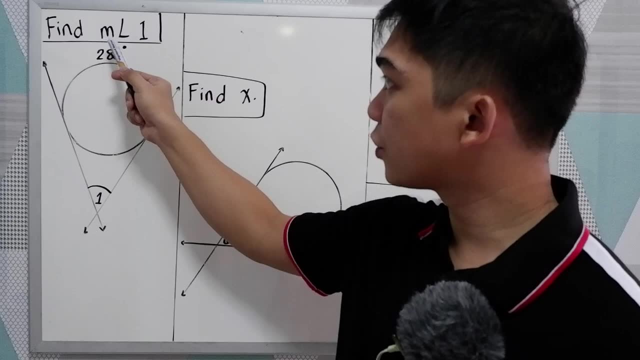 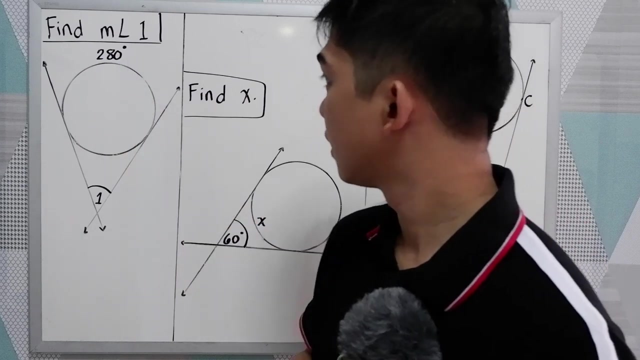 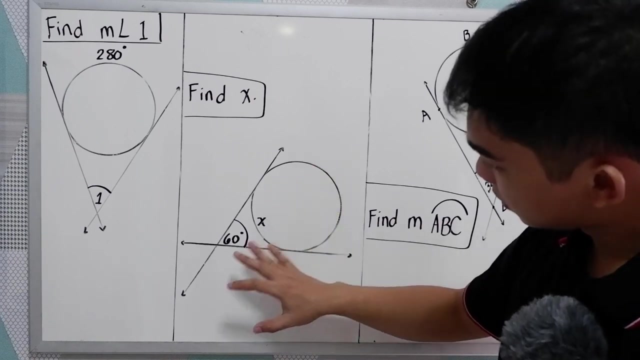 Now, to better understand our fourth theorem, let us try to solve the following problems. In our first illustration we are going to find the measure of angle 1. Given the arc 280 degrees, And for our second illustration we have 60 degrees as our exterior angle. 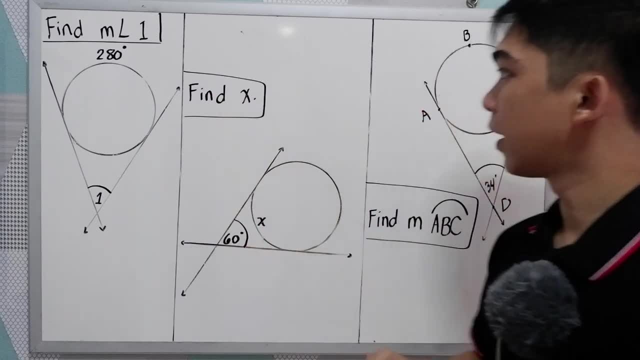 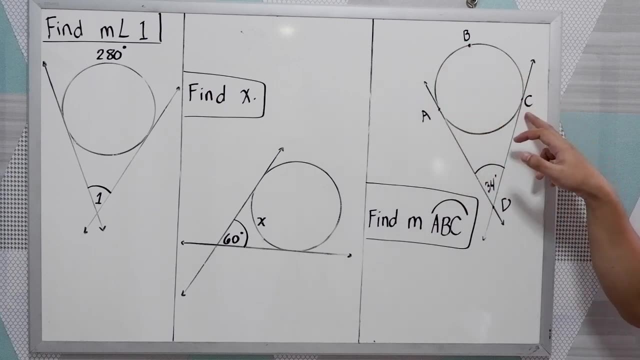 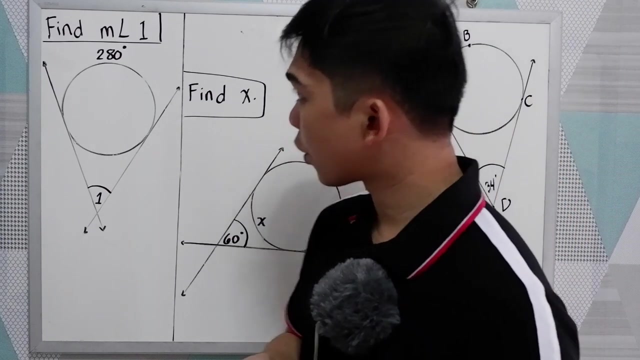 We are going to find X And in our third illustration we are going to find the measure of the arc ABNC, Given the exterior angle. So we are going to apply the theorem number form to get the unknowns. So let us try to solve number 1.. 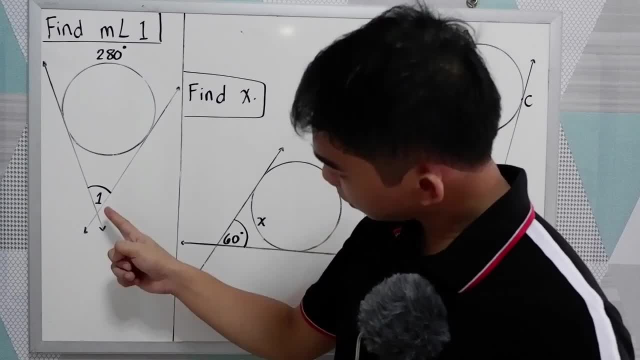 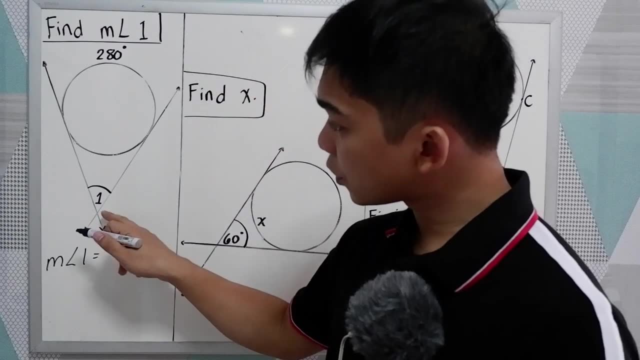 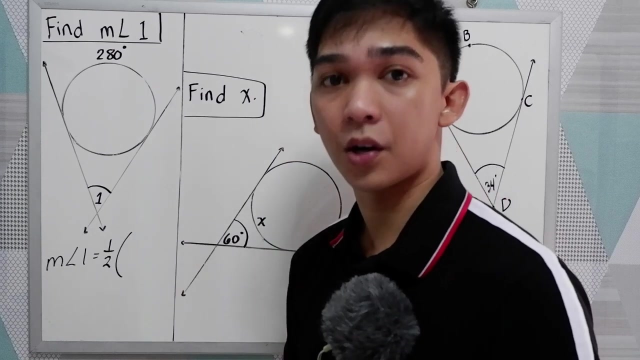 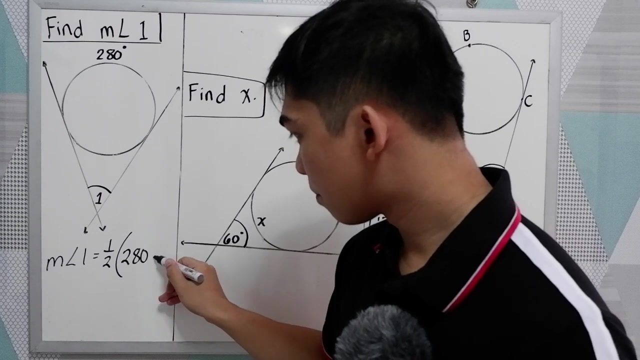 Find measure angle 1.. So angle 1 is here, So we need to find measure angle 1.. We know that the measure of the exterior angle is one-half of the difference of the intercepted R, So we have 280 minus. 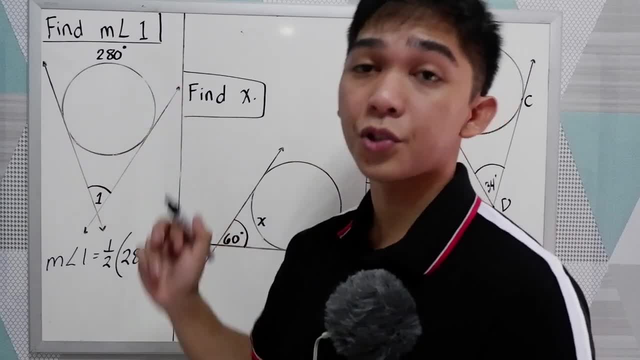 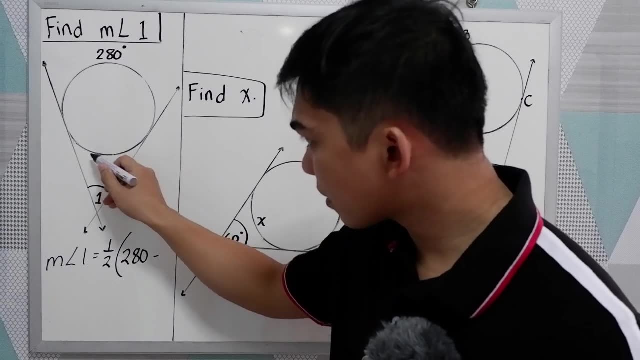 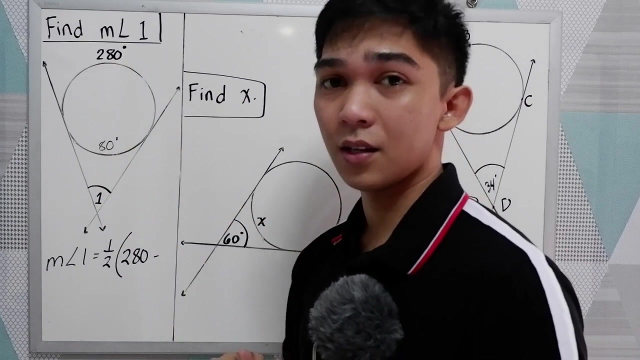 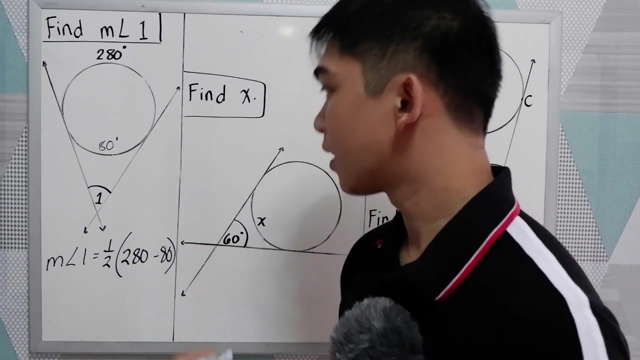 We know that one revolution is equal to 360. So this arc measures 80 degrees. Why? Because 280 plus 80 gives us 360. So 280 minus 80. That would be our arc, So one-half. 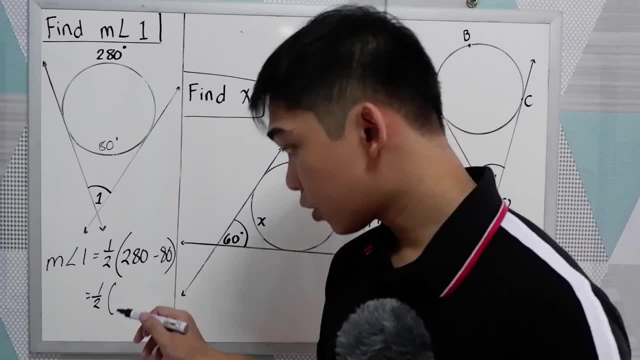 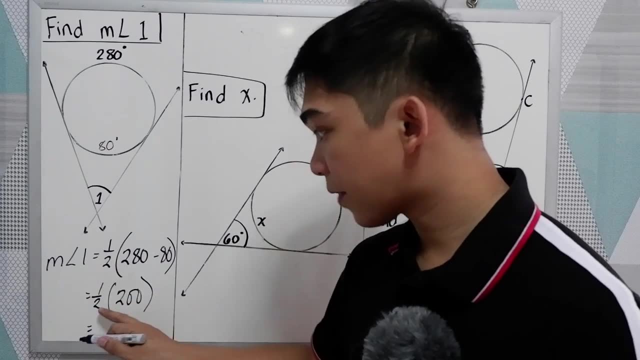 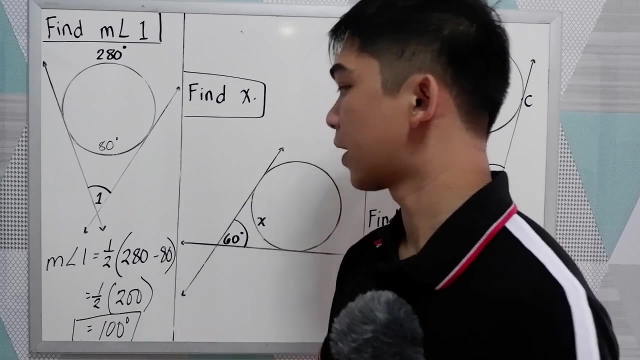 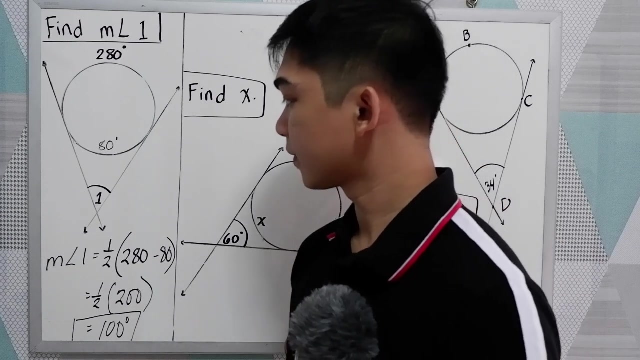 280 minus 80.. That is 200.. Now to get the measure of angle 1.. 200 divided by 2.. So this is 100 degrees. Okay, The measure of angle 1 is 100 degrees. Let us proceed with our second problem. 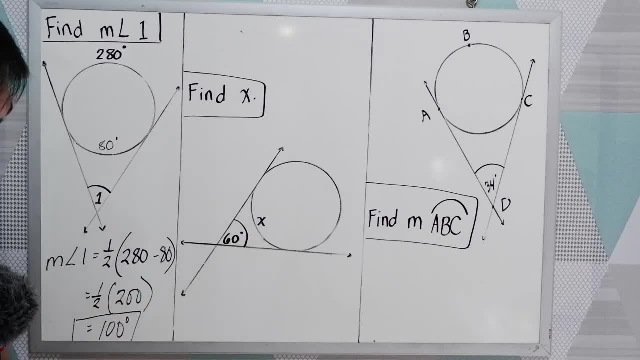 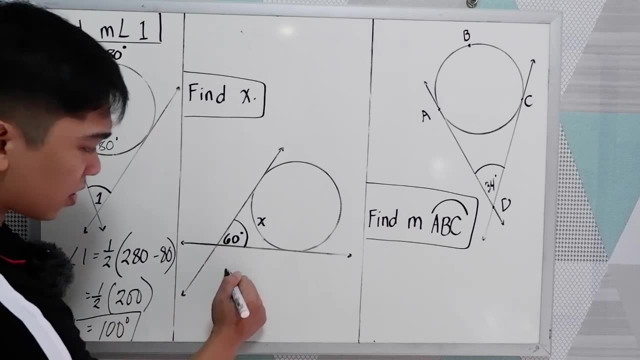 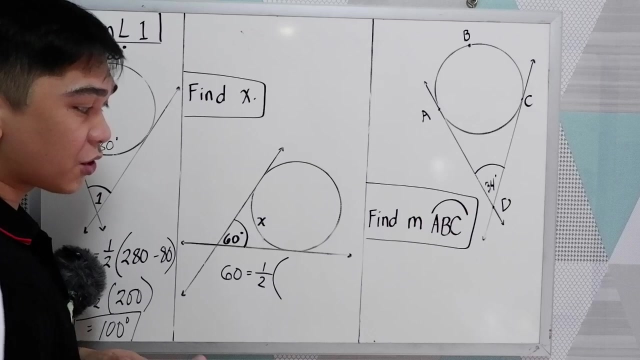 We are going to find X, X, Given the exterior angle. In this case the exterior angle is given, So 60 is equal to one-half. The exterior angle is equal to one-half of the measure of the intercepted arcs Minus. 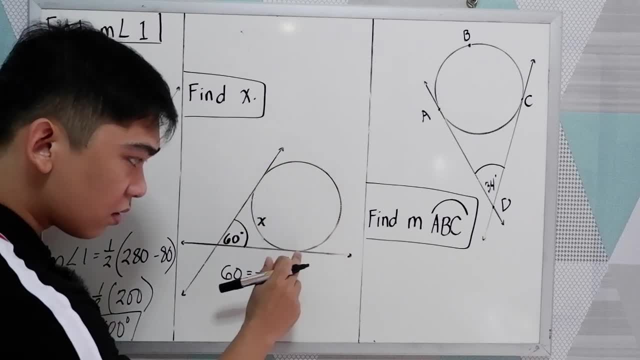 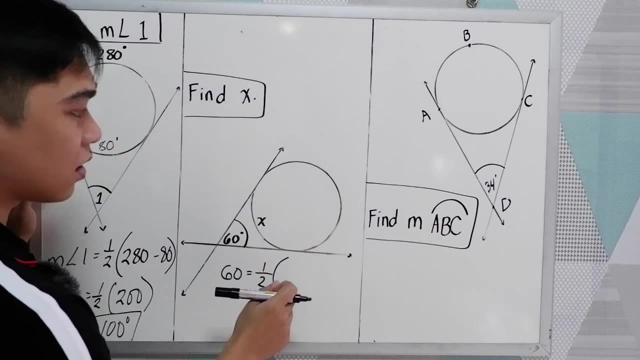 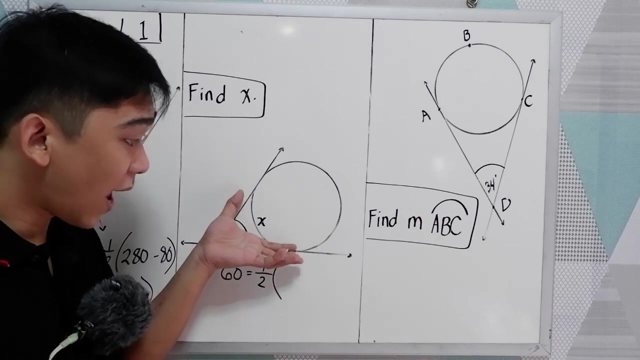 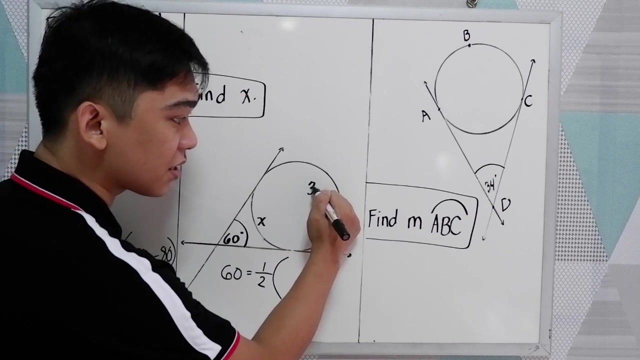 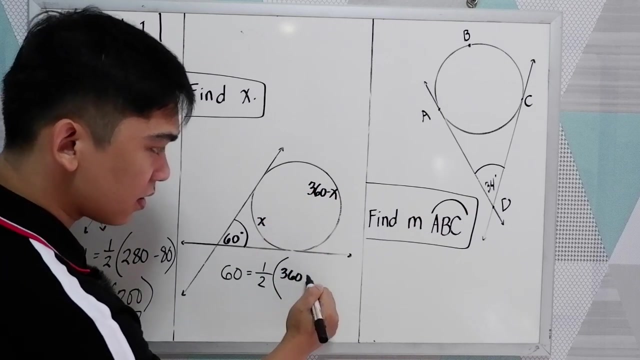 So the bigger one, We can get the bigger arc using the definition: One revolution is equal to 360. So if this is X, we can get the measure of the bigger arc. So that is 360 minus X. So 360 minus X. 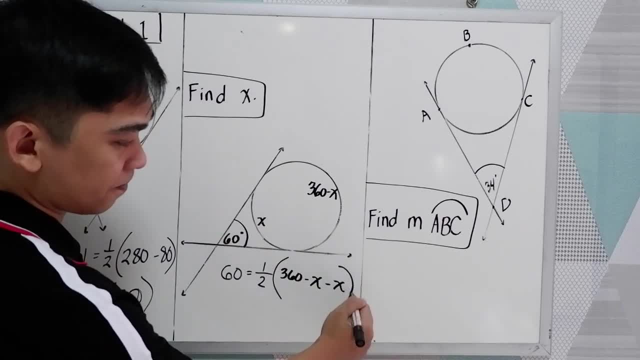 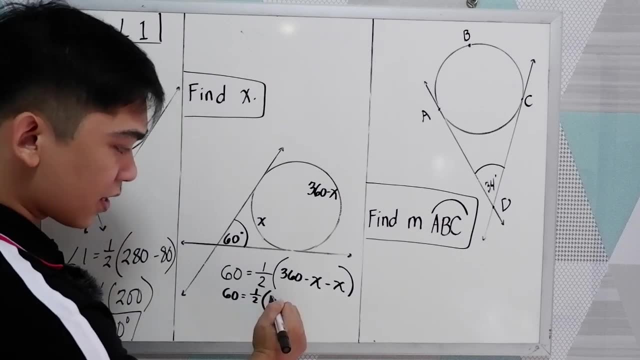 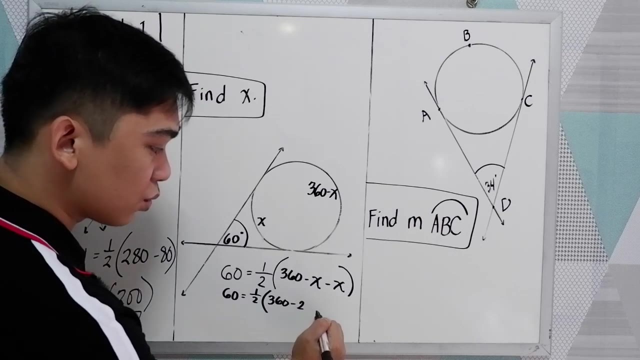 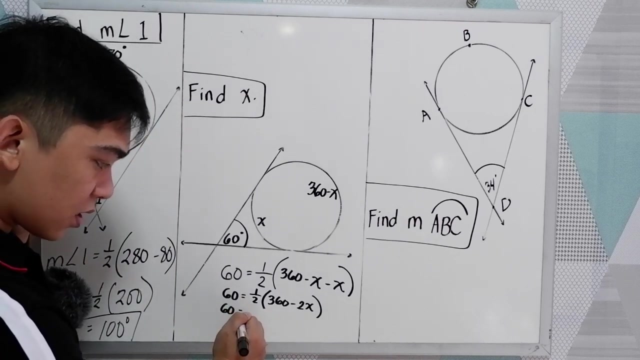 We need to subtract the second arc minus X, So we have: 60 is equal to one-half of 360.. Negative X minus X, That is negative 2X. Okay, Now we have 60 is equal to Distribute. 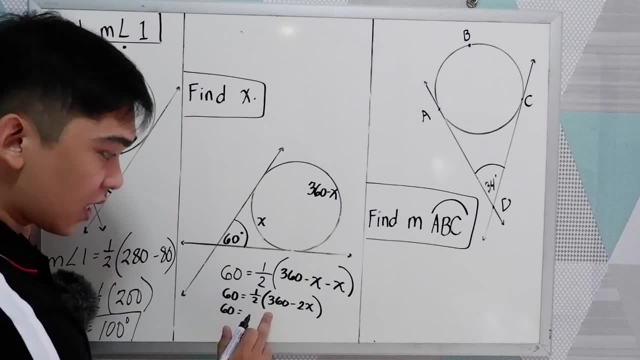 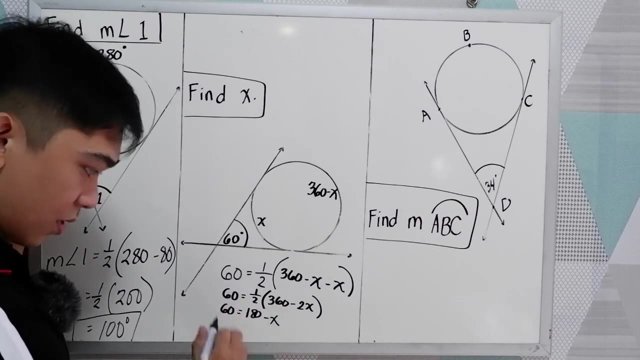 So one-half times 360.. Basically, that is 360 divided by 2.. So 180.. Minus one-half times negative 2X, That is negative X. Now X is equal to 180 minus 60.. 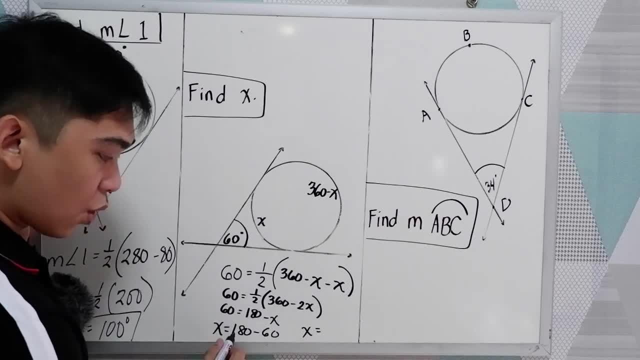 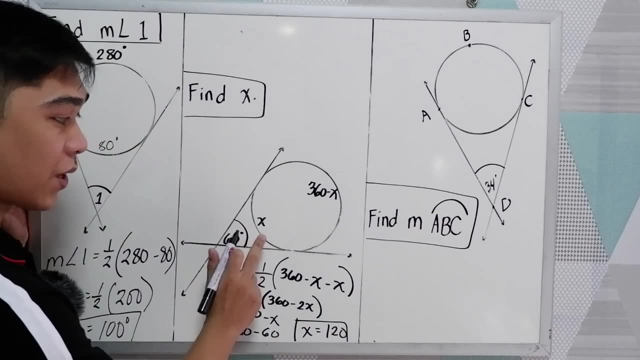 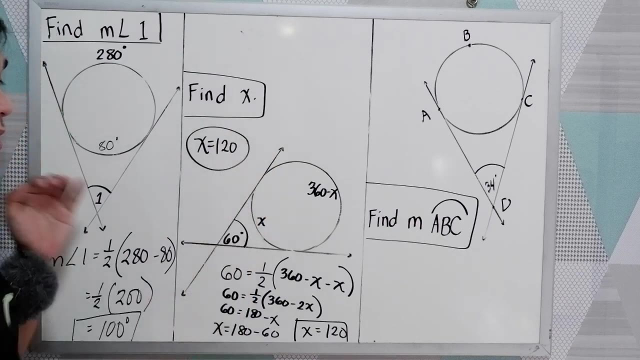 So X is equal to 180 minus 60.. We have 120.. So the value of X here is 120.. So X is equal to 120.. Now to get the measure of the bigger arc, So 360 minus 120.. 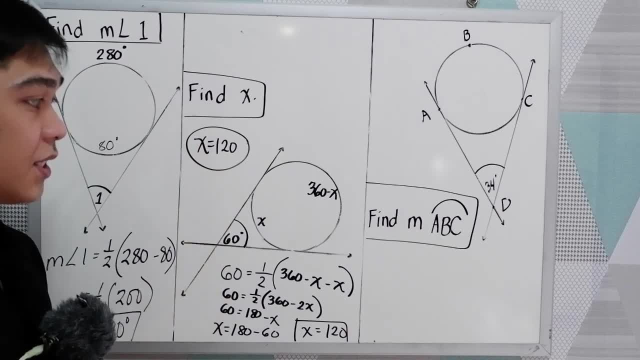 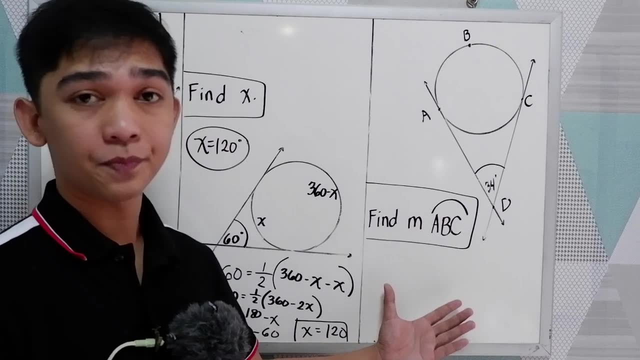 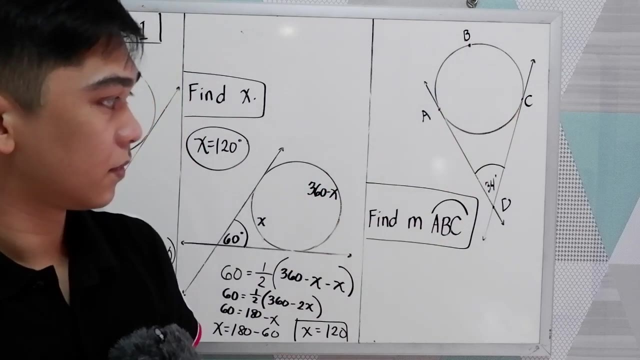 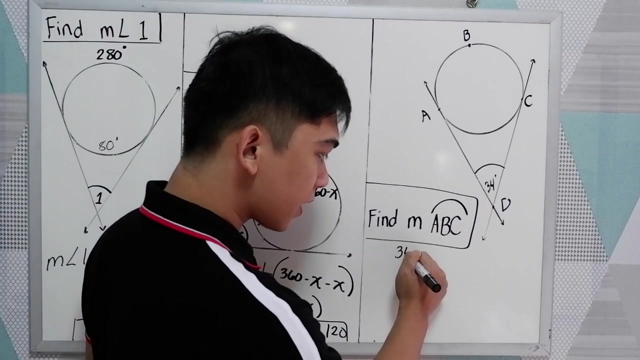 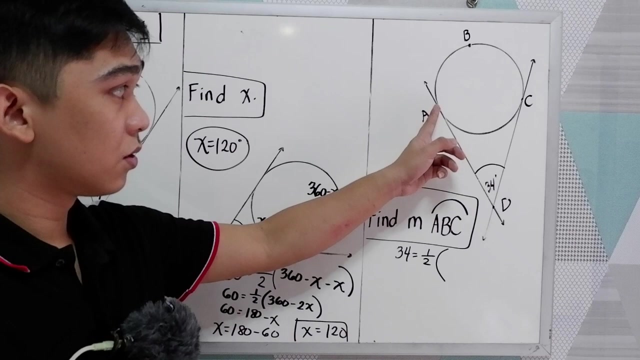 That will give you 240 degrees. And for our third problem, we need to find the measure of arc ABC, Given the exterior angle, which is 34.. So the exterior angle 34, is equal to one-half of the difference of the intercepted arcs. 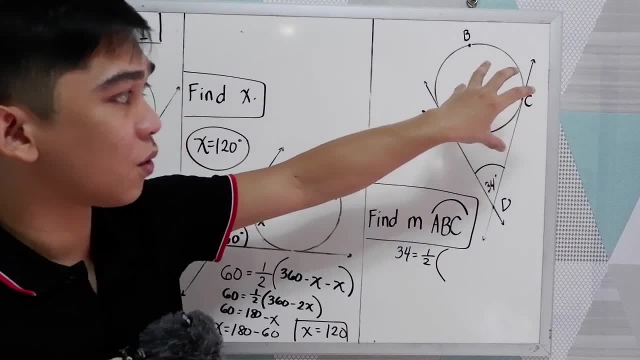 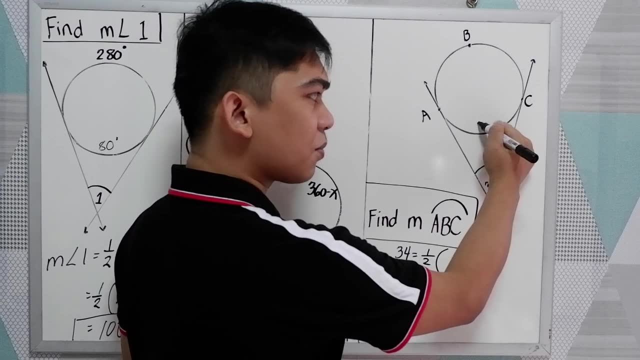 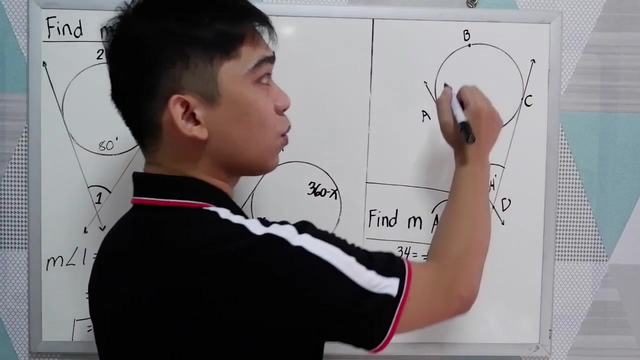 So in this case we don't have a measurement for this, So we're going to assign AC as our Let's say. let's use the variable A, So AC will be our A. Therefore, the bigger arc is equal to 360 minus A. 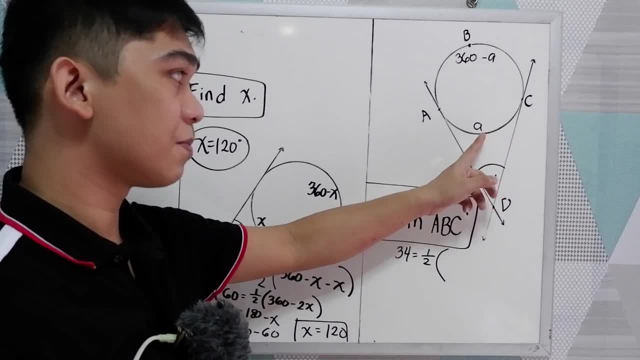 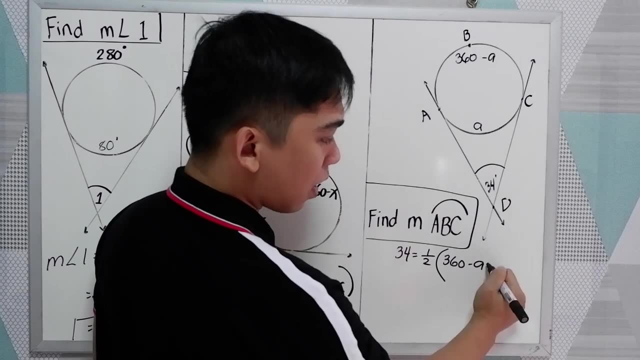 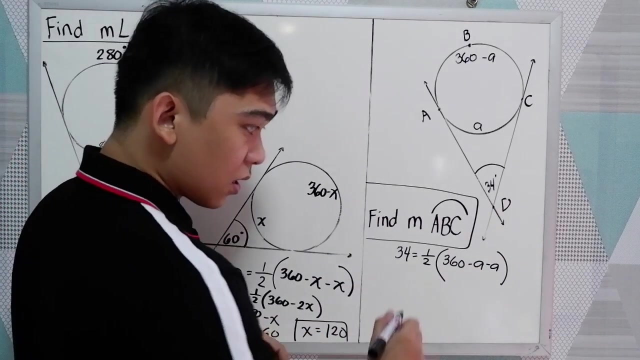 If you want to use X, that's okay. If you want to use B, okay. So we have 360 minus A minus A. The same process with number 2.. We're going to find the value of A first. 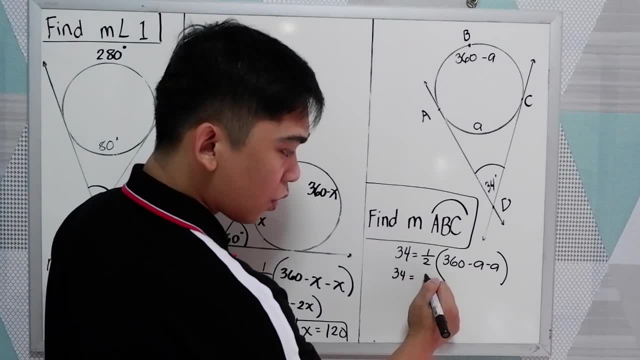 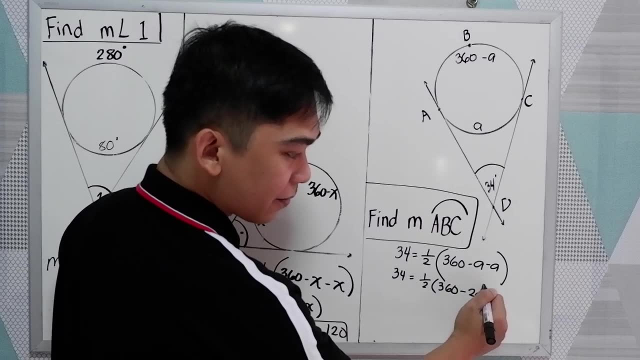 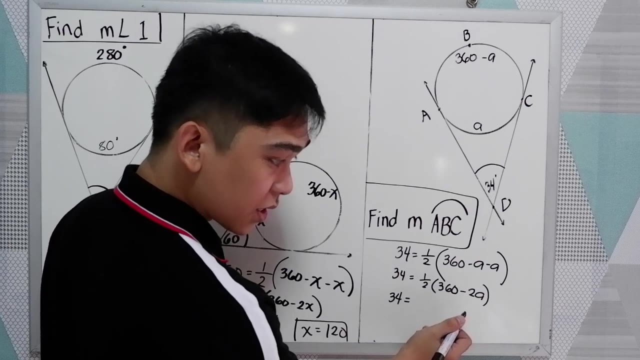 So we have: 34 is equal to one-half times 360, negative A minus A negative 2A. So 34 is equal to one-half times 360.. So that is 180.. Minus one-half times 2A.